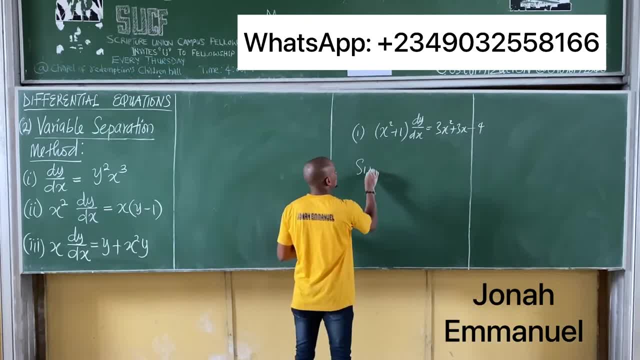 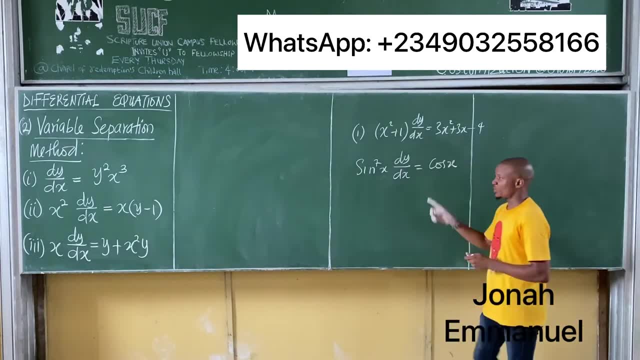 I had something of this nature: Sine over 7x, The y over the x, equal to cos x. See the difference between this one and this one. In this one here, observe x and y are not mixed. This is just in terms of. I have just one variable here: x. 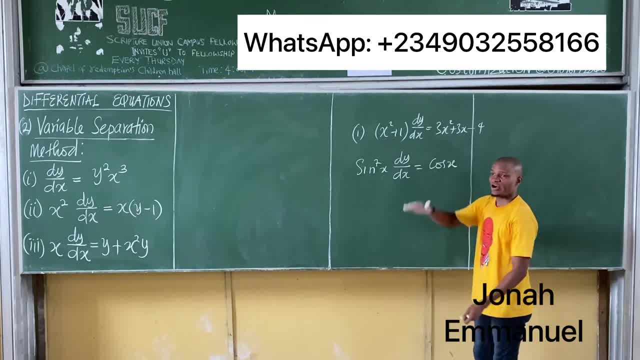 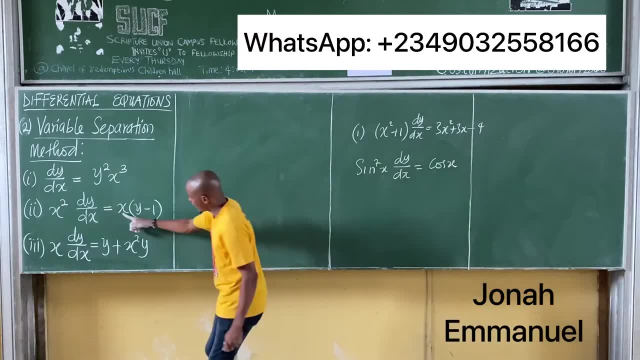 I have just one variable here: x. Same thing here. Check all the examples we did. It was just one variable, One variable, That's x and x. That was it. But in this case- now observe, it's now x and y mixed. 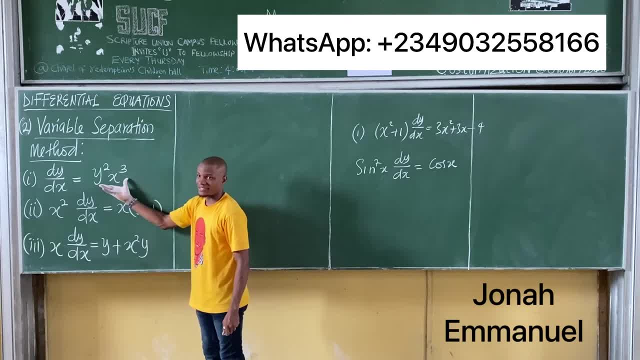 It's now x and y mixed. It's now x and y mixed. At this point, now, it's no longer this method, Now it becomes variable separation. Please, you must be disciplined, Because in terms of exam, they won't say using variable separation. 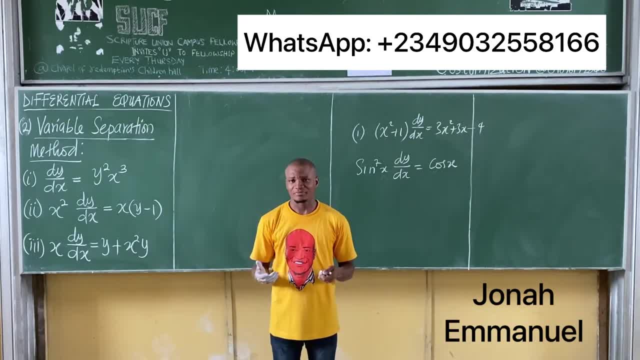 They won't say using direct substitution In terms of exam. they won't say using direct substitution. They won't say using variable. They expect that you should know. And how do you know? By looking at it with your depth: If I have two variables mixed, it's variable separation. 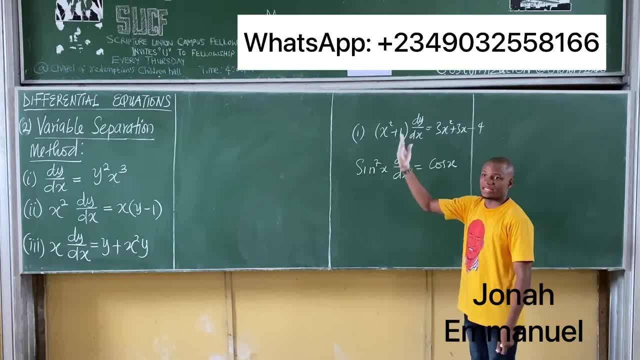 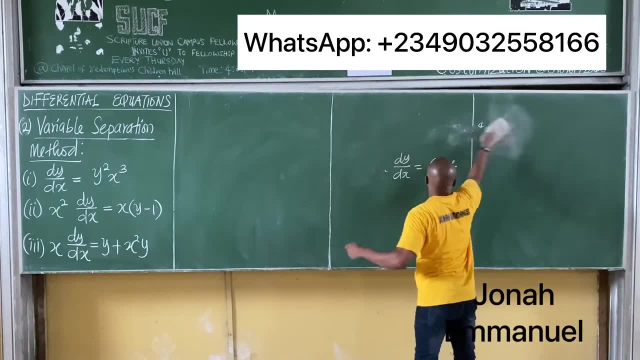 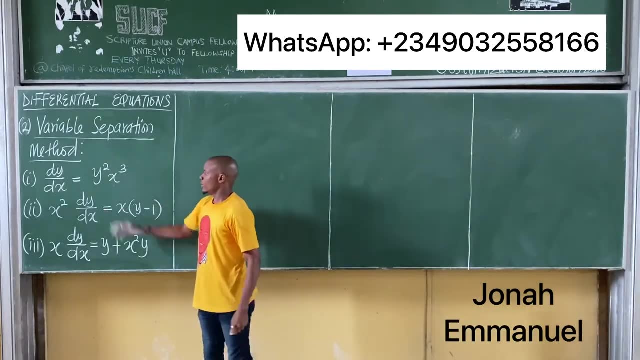 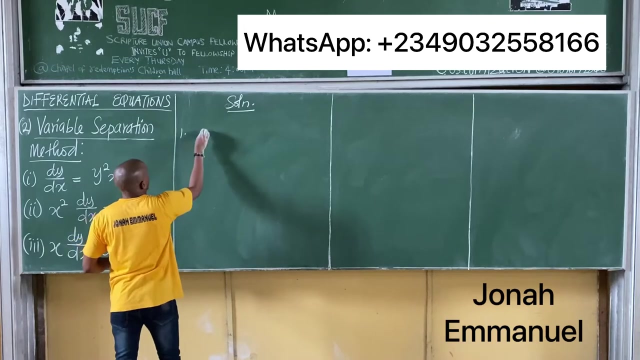 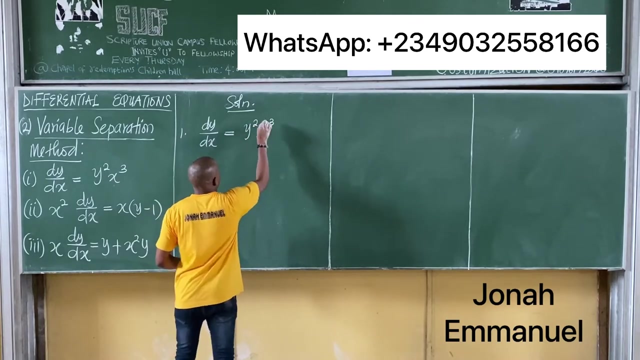 If I have just a singular variable, it's direct substitution, And that's like that. Alright, Let's solve this distribution. The first case: I have number 1.. I have that the y over the x is equal to y squared x over 3.. 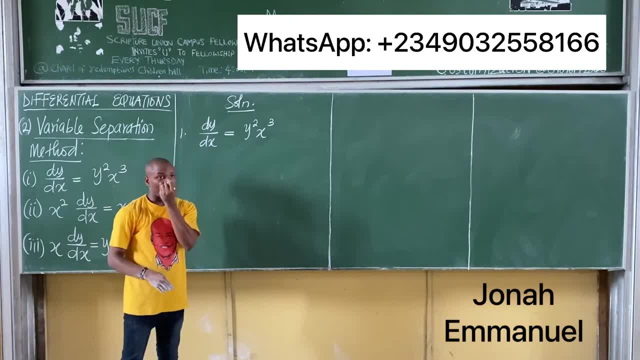 In this case, observe x and y. In this case, observe x and y are mixed. So what next In this case? now, what I have to do is to do separate separation. Move x to your right hand side. Keep y on left hand side. 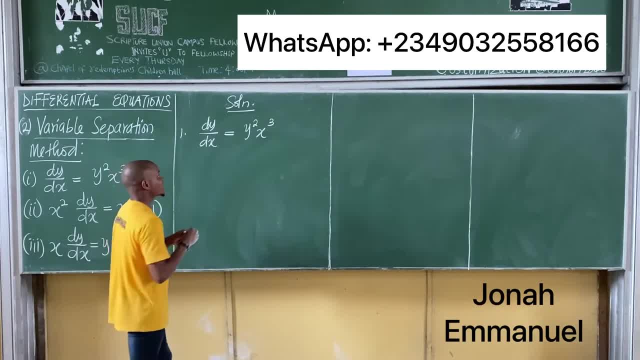 How do I do that? My first task is to move this man over here. Of course, this one here is all about 1.. Such that 1 times the y is the y. So I have that the y times 1, which is the y, is equal to 1.. 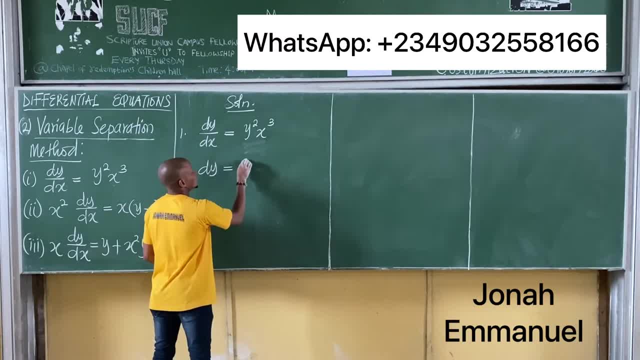 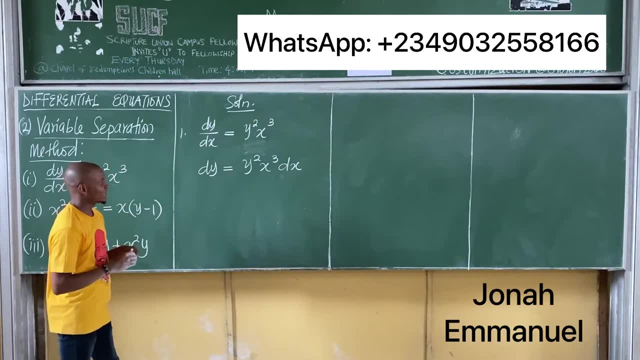 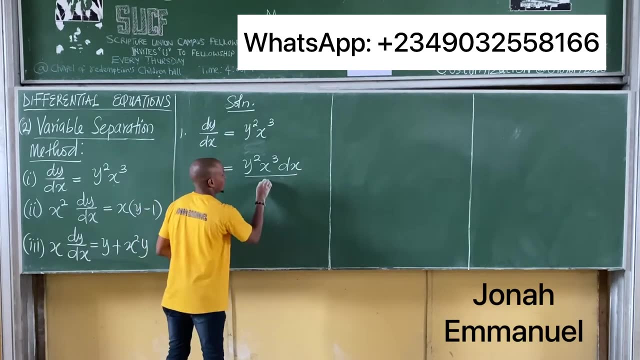 This times this: That one gives you y squared, x cubed. Relax, I have it. So what next? I still have to look for a way to bring y over here. What I like to do is as easy as dividing by water: y squared. 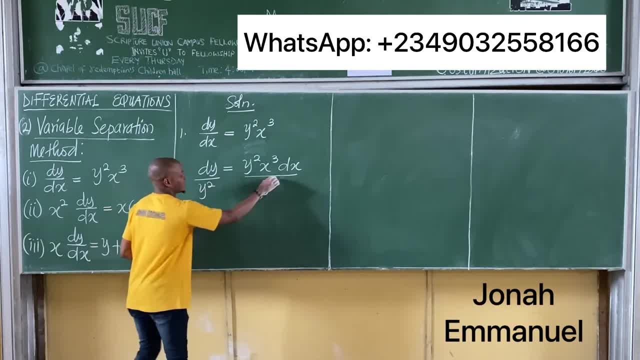 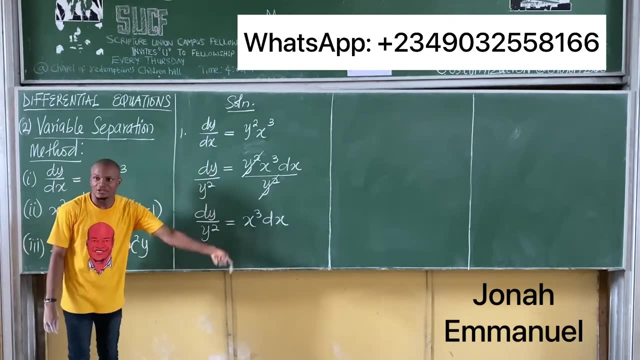 Dividing by water y squared. This cancels this. I'm now left with the y over. y squared is equal to y squared. This is equal to x cubed dx At this point now. I have now done the variable separation. 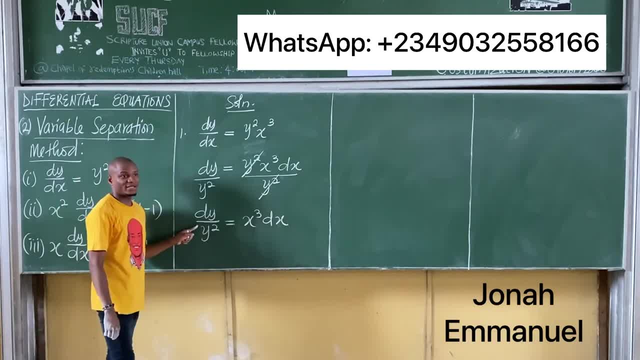 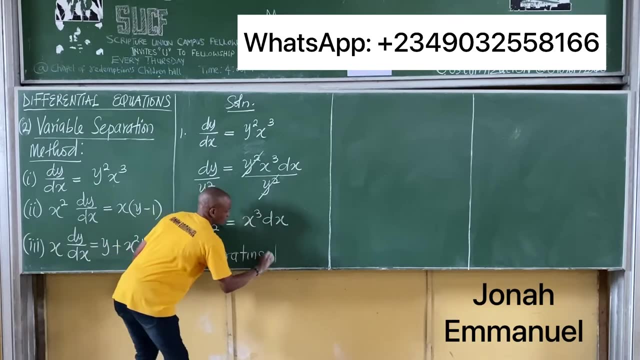 I have moved everything that concerns y to my left hand side. I left everything containing x to the right hand side. That is At this point now. I can now integrate, So hence, integrating through, Integrating through. If I integrate through, what do I get? 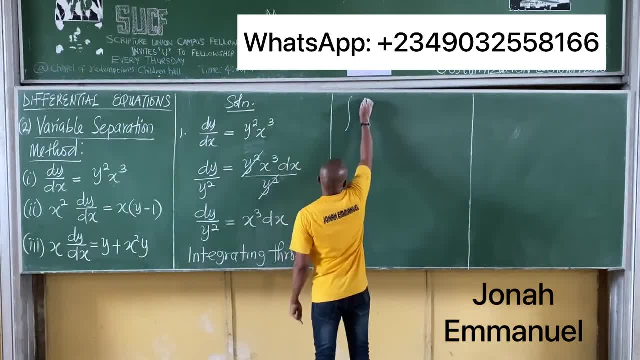 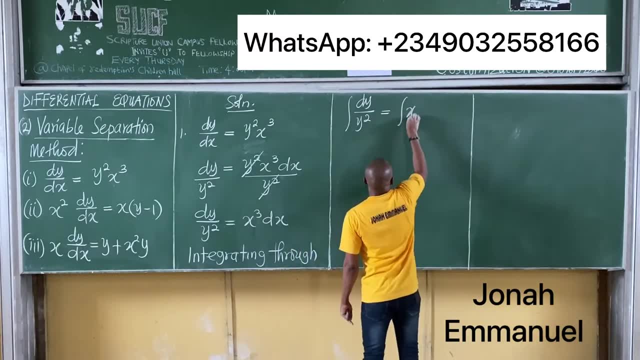 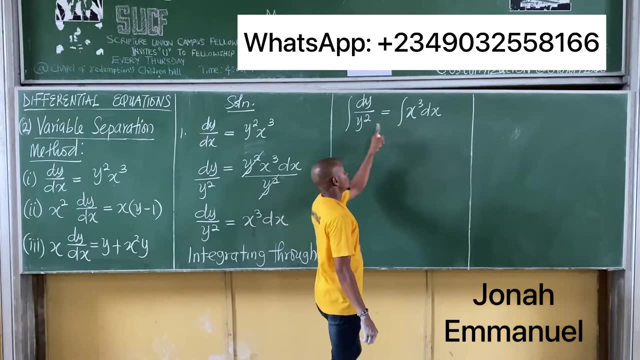 I have that it integrates. I have the integral of this one here. The y over y squared is equal to the integral of x cubed dx. This one is easy to integrate And it's a general method In this one here. what do I do? 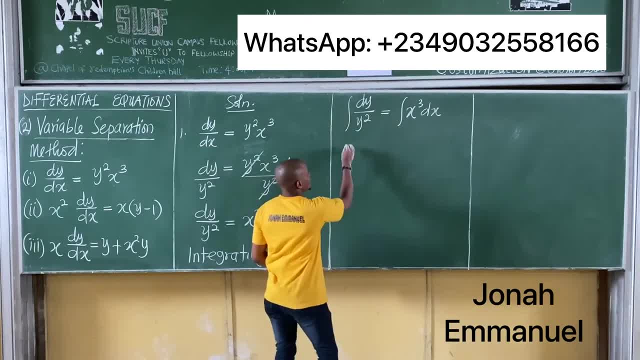 Your idea would be this: Shift the y out of this, So I'll be having the integral of. If I move the y here, I'm having 1.. So it becomes 1 over y squared dot y, And these two are the same thing. 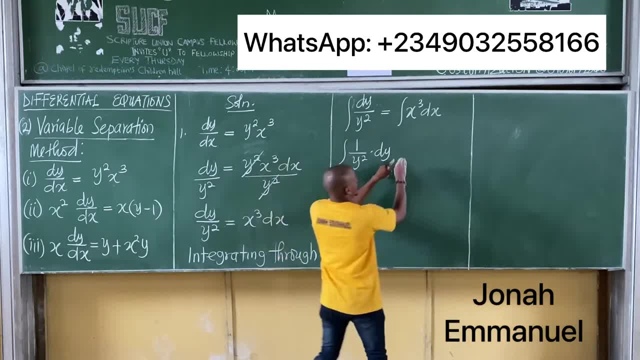 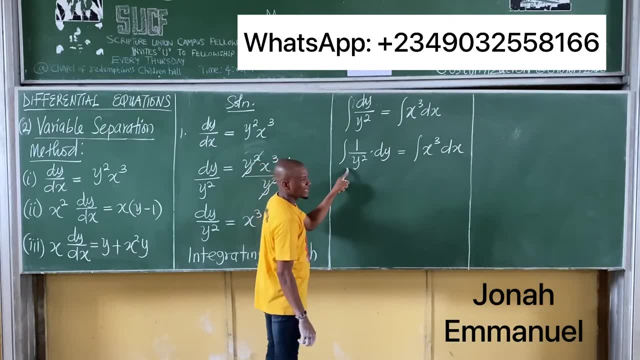 Of course 1 times the y is the y over y squared Is equal to the integral of x cubed dx. If I move this one here, observe This will not be mean Why This one here is not 1.. 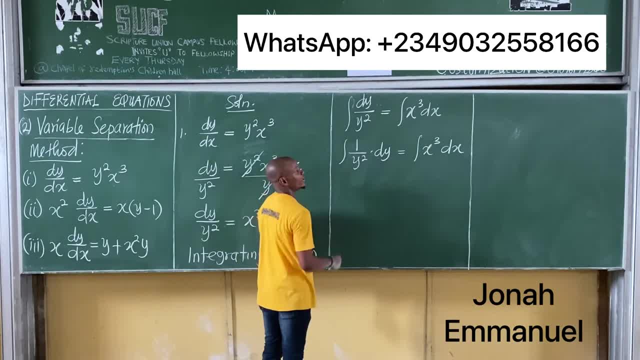 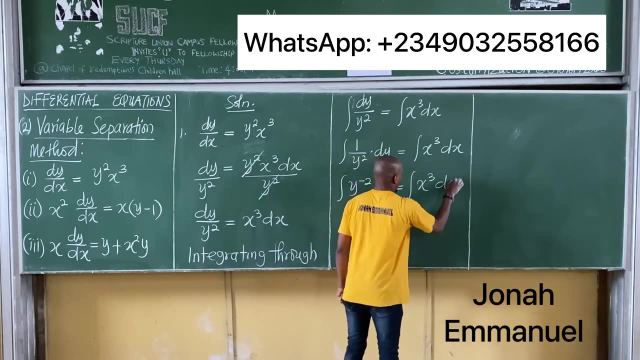 So you can't be mean. So what do I do here? now Express this one here in terms of index form. So it becomes the integral of This. one becomes y over there minus 2 in index form. Next one: The y is equal to integral of x cubed dx. 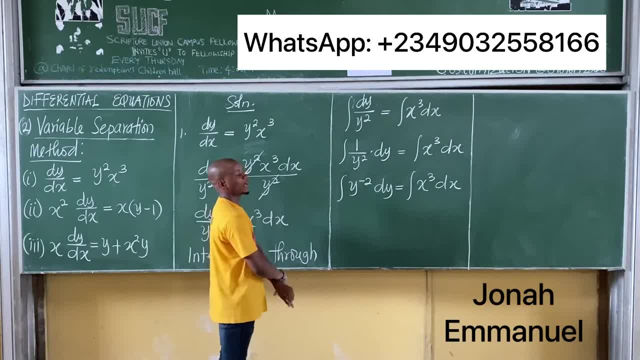 This one now looks easier to integrate. So for these two here I can now use general method, Which means add 1 to the power And divide by what you have here. So to this one it becomes y minus 2 add 1.. 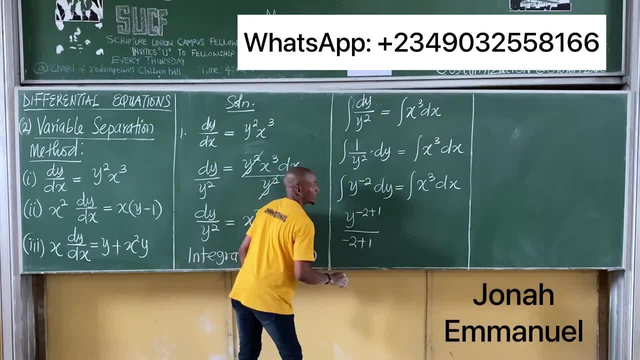 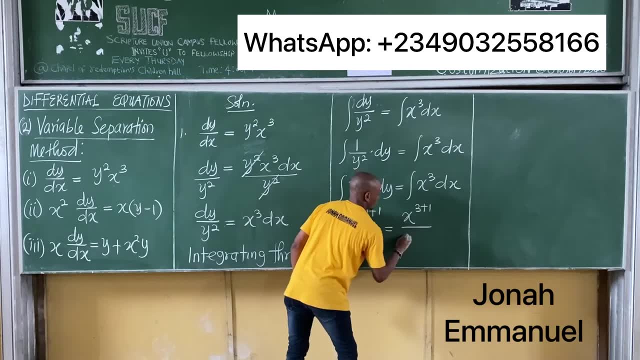 All over what I have here: Minus 2, add 1. Is equal to this one here: x3. add 1 to this Plus 1. All over 3 plus 1. Plus 6.. So I have this. 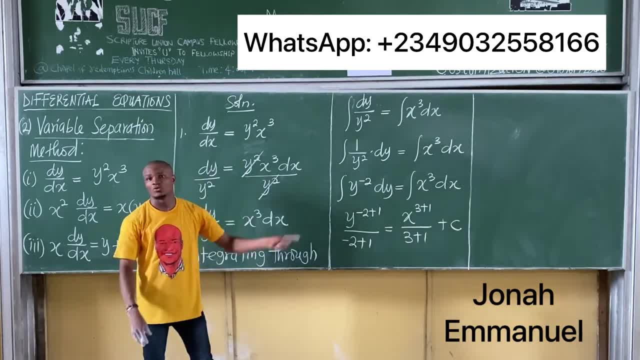 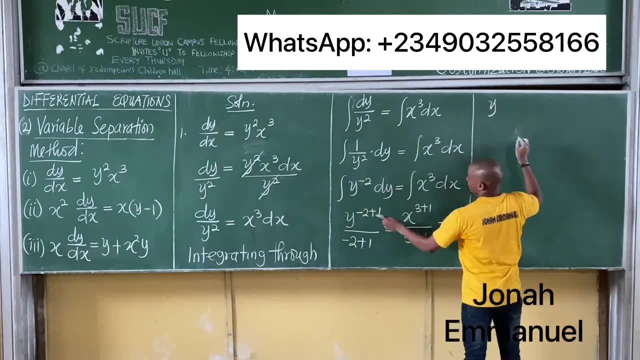 Right, So I'm done Just before I make the simplifying. I'm done, So simplifying is what I get. This gives you y Into minus 2 plus 1.. Minus 1. All over, minus 2 plus 1.. 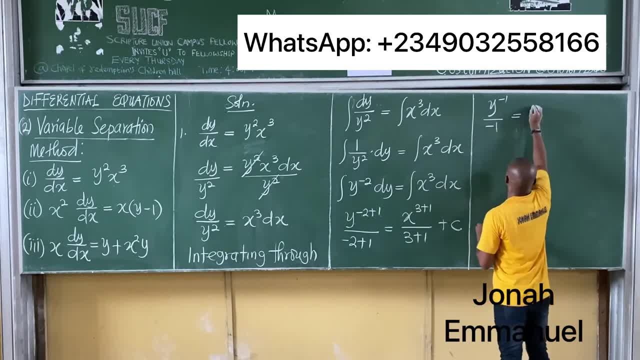 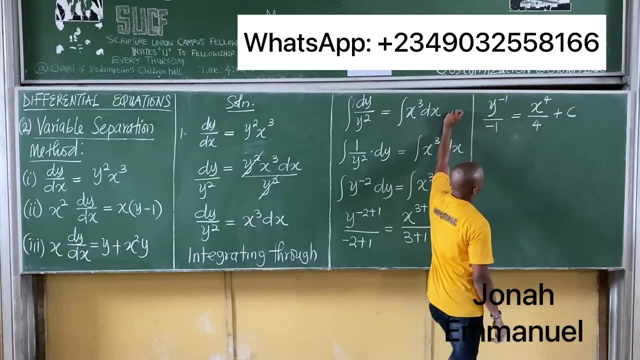 Minus 1. Is equal to x into 3 plus 1.. 4. All over 3 plus 1.. 4. 4 plus c. So I have this. This one is not okay that much. So look for a way to simplify to our product. 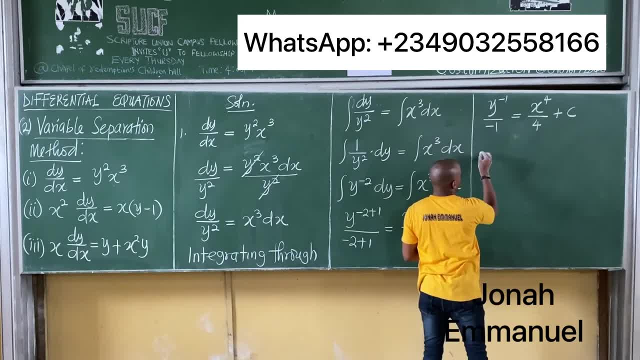 What do I get there? This one becomes: Look up here, This one here, Because I set sheep's one out. I have one here. So sheep's has become 1 over minus 1.. Multiply y by minus 1.. Because 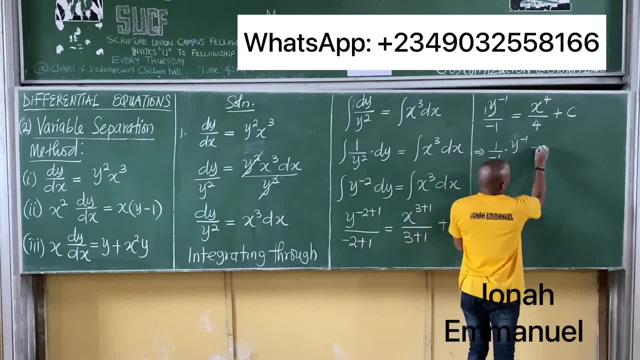 I guess if you move this one outside, It's equal to This: gives you 1 over 4 x. Yeah, 1 over 4 n to the power 4. Plus c. So listen, This piece here don't really matter. 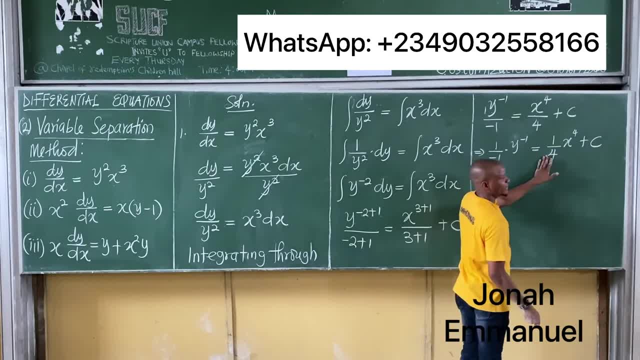 You ask me Because, Don't forget, we said, When it comes to doing, What do you call it Differential equation? The idea is this: I want to express this man From y by x to y. I should have stopped here. 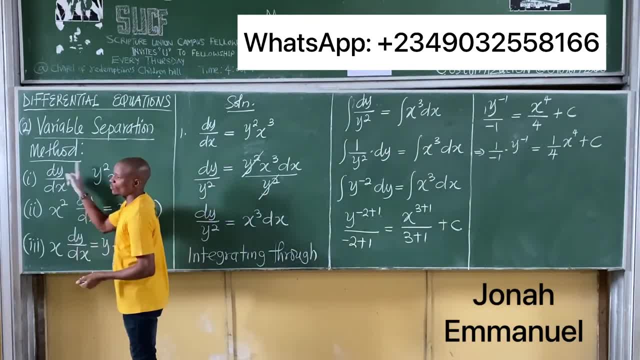 If I stop here, It's not that bad. But the thing is this: I want to get y, Not in. I want to express this man From y by x to y. I should have stopped here If I stop here. 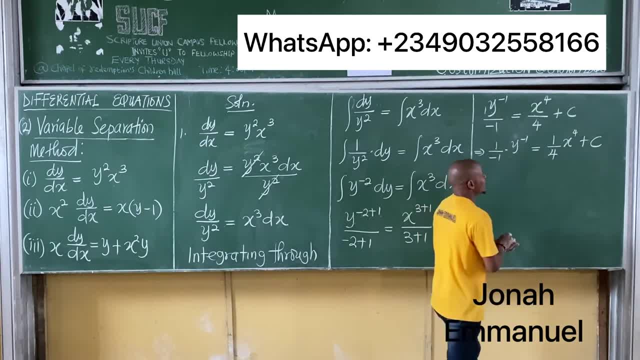 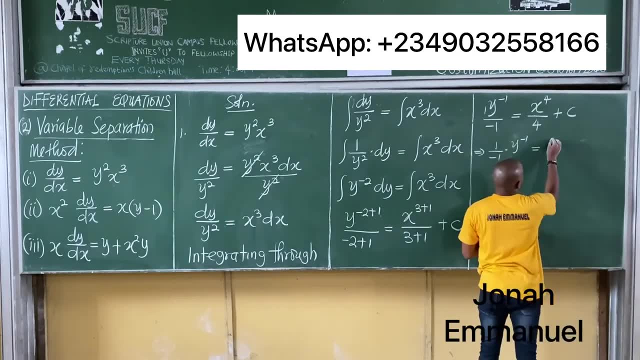 It's not that bad, But the thing is I want to give y, Not in. That's why. So, if I leave x In this form Back to this, More like saying Don't really care about x, x already sent me. 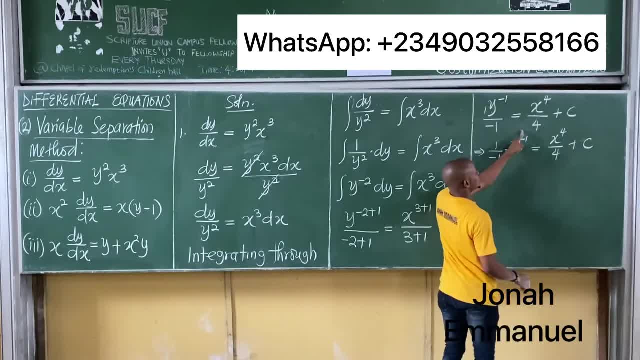 No problem about x. The problem is Not: now I want to get, I want to make y. So For the formula, Of course, This is Minus 1 over 1.. That gives you Minus 1.. 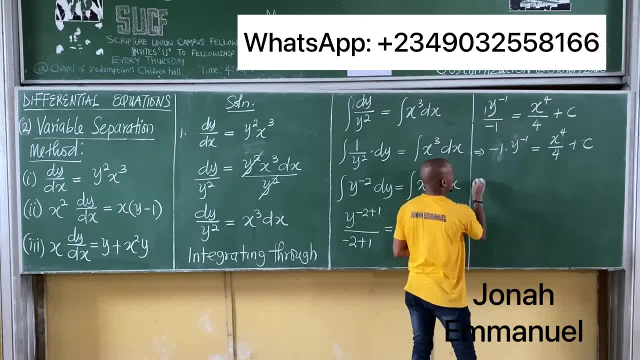 So Here becomes Minus 1.. Express this one. This will now give you What I will get here: Minus 1. Y over 1.. Minus 1 is what there, 1 over 1 is equal to F over 4 over 4 plus C. Minus 1 times 1 gives you minus 1.. This is going to give you minus 1.. This answer is fine, No problem. 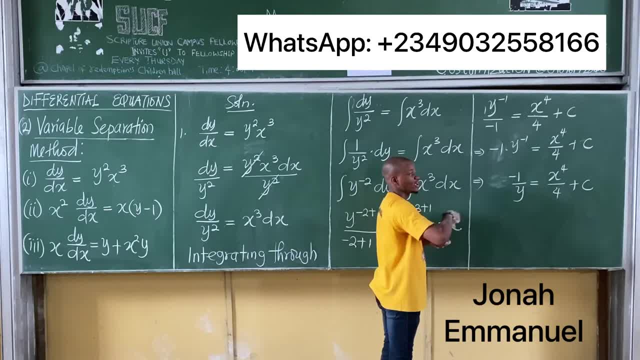 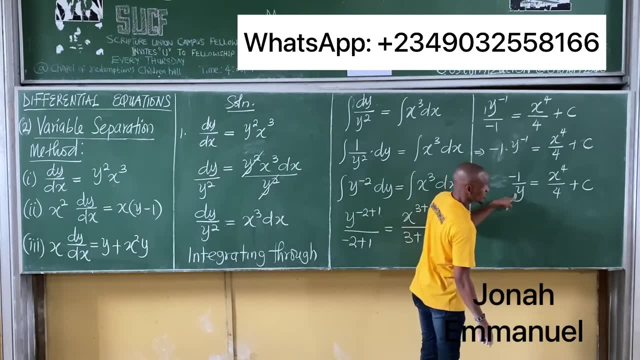 But then in differential equation. in differential equation, my task is this: Make y circle to the formula, Not inverse of y, Not negative inverse of y. My task, my idea now would be this: How do I make y here circle to the formula? What do I do? 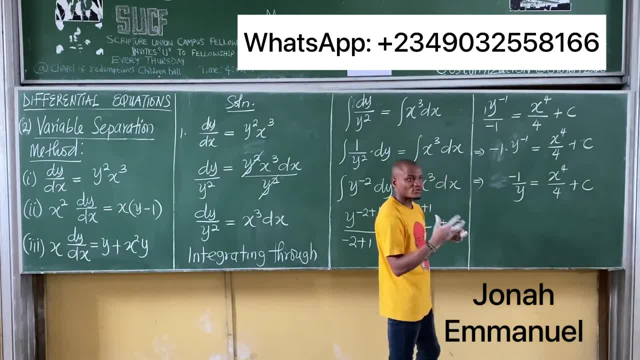 I want to make y here, to stand in the loop. What do I do? Divide by what? Divide by minus 1.. If I multiply it by my 2, it becomes minus 1. like this, It becomes plus 1.. It's not y, So it becomes 1 over y. 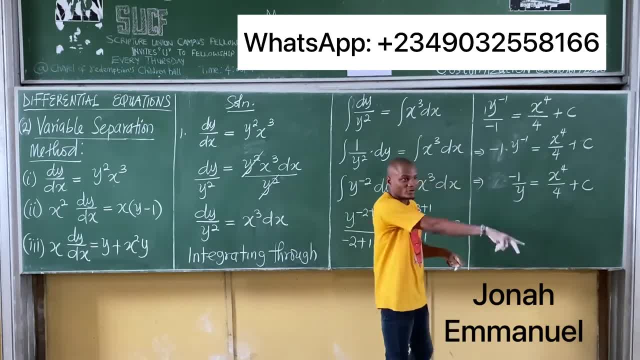 My task is this: I want to make y to stand in the loop. What do I do? Divide by minus 1.. So my task now would be this: This is now equal to minus 1 over. y is equal to before it goes into black. 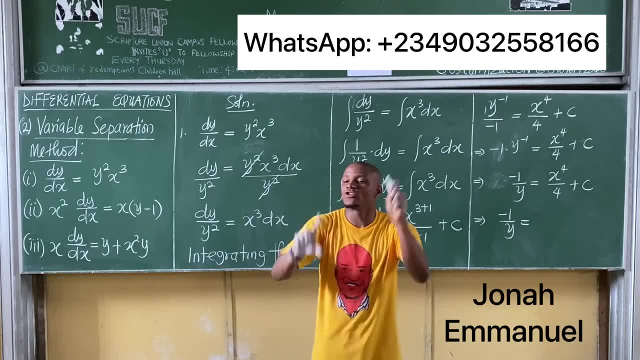 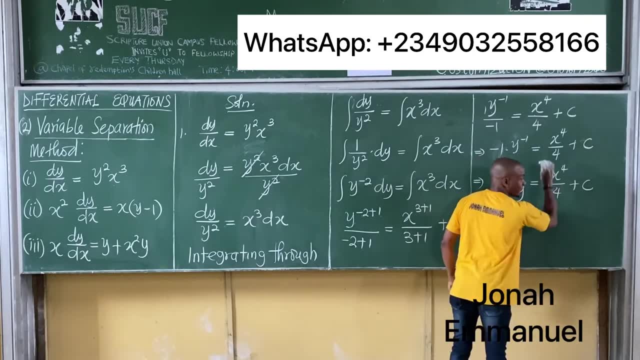 we should know that you don't. You don't cross multiply 2 fractions if they are not whole. Before it cross multiply, we must make this one whole first. So the idea is 5 MCL here first, That will now be 4.. 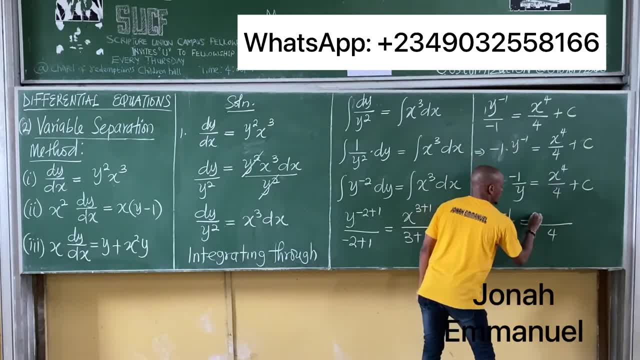 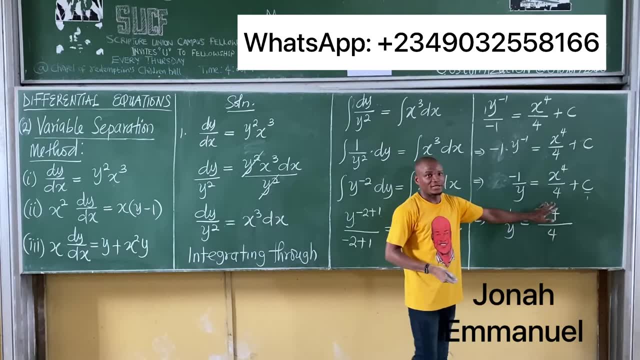 4 over 4 is 1.. 1 times x power, 4 is x power 4.. Plus, this is 4 over 1.. This part, This part is debatable. Listen, This part is debatable, So others say: 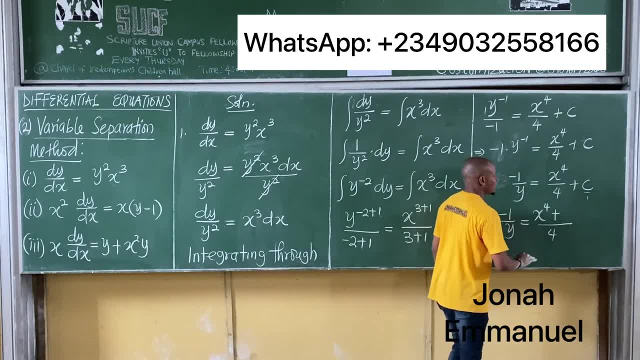 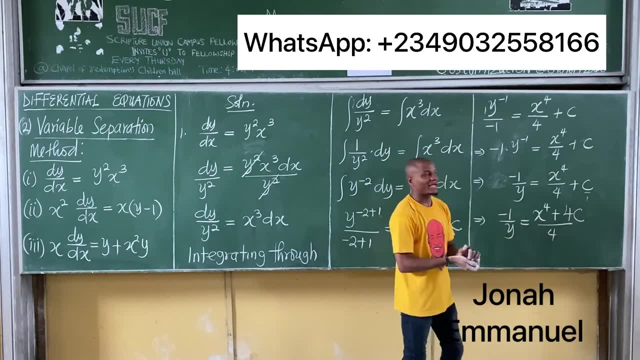 Now, usually, if I do it this way, it should be 4 by 1, that's 4, like C, 4C. so it has to be 4C. Some authors would be like, don't worry about the 4C, that means you only see. some authors would just only see like this: 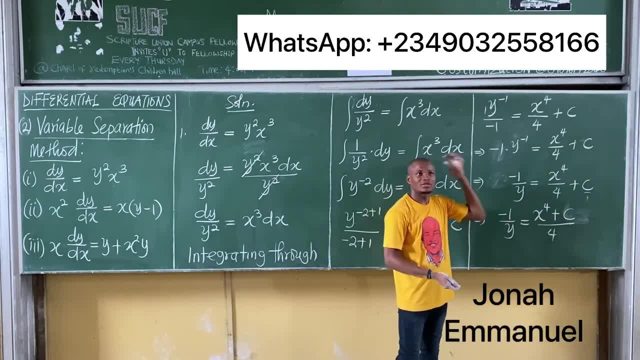 Now, if I have done it before, what is a constant? that's how it works. the constant is unknown, So you don't have to do 4C. some authors just use C, not the usual 4C. So whether you do it this way or 4C- depending on who is marking- 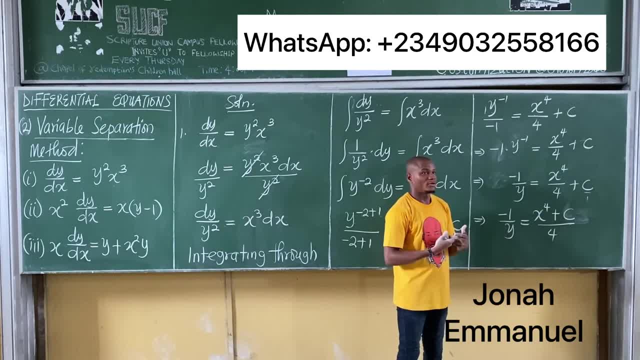 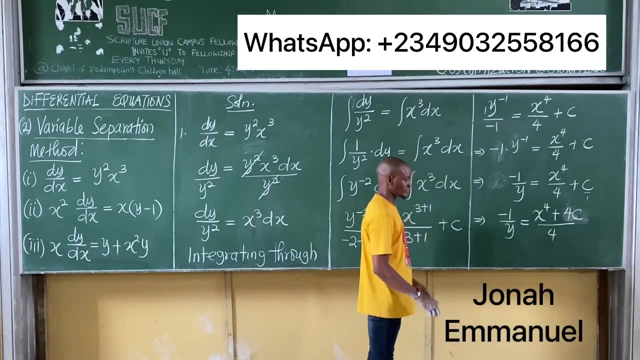 So yeah, depending on who is marking, Let's not do the normal stuff. I think I pointed out something here, but let's do the normal stuff. Normal stuff is going to be 4C. are they 4C At this point? now listen. 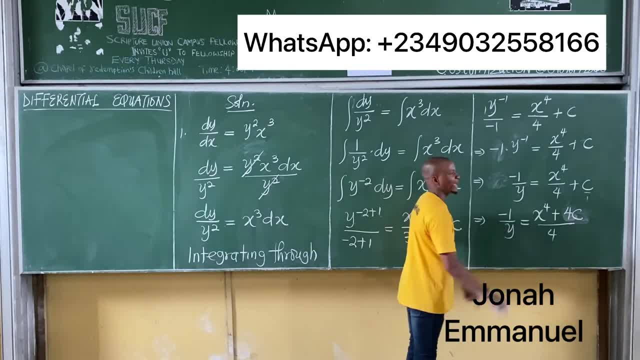 At this point now, listen, At this point now, I can now cross-multiply. Why I have just a singular fraction and a singular fraction. you don't cross-multiply, except you have singular fractions. So at this point, yeah, it's not proper for me to cross-multiply. why? 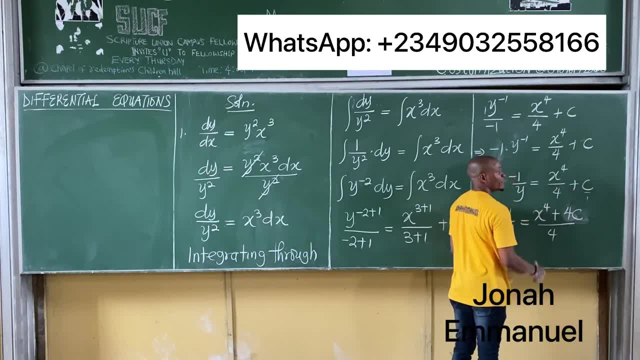 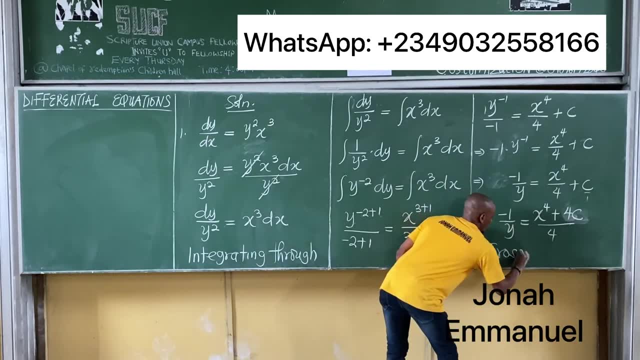 This is not a singular fraction. I have a fraction and a constant. If I cross-multiply, leave them one, as in this case, right Before cross-multiply. So at this point now, cross-multiply, Cross-multiply. 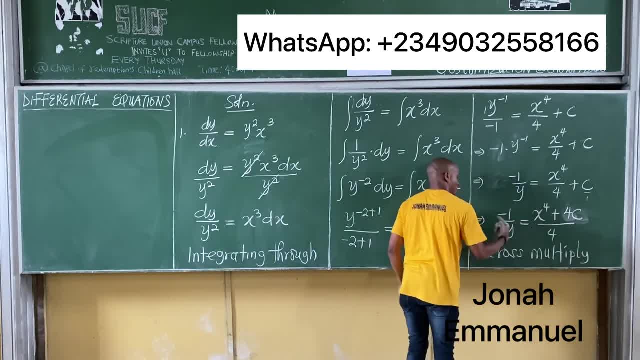 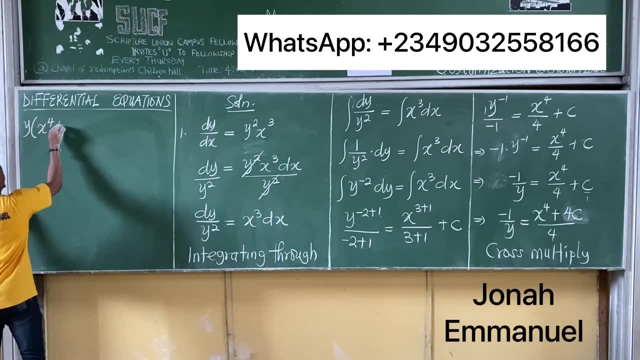 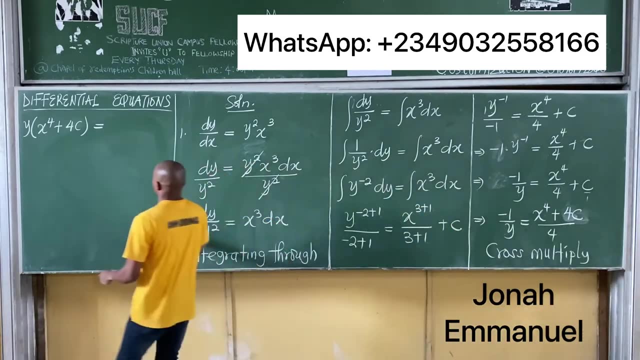 Cross-multiply. This one comes here. This one comes here. So I'm having Y Y into X to the power. 4 plus 4C is equal to this times this Minus 1 times 4, you see what's there. 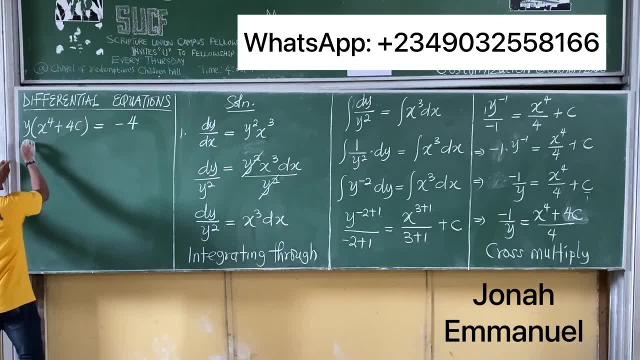 Minus 4.. Finally, get Y. I will now divide that by X to the power 4 plus 4C. Divide that by X to the power 4 plus 4C. This one will now come to this. So hence I have that Y is equal to minus 4 all over X to the power 4 plus 4C. 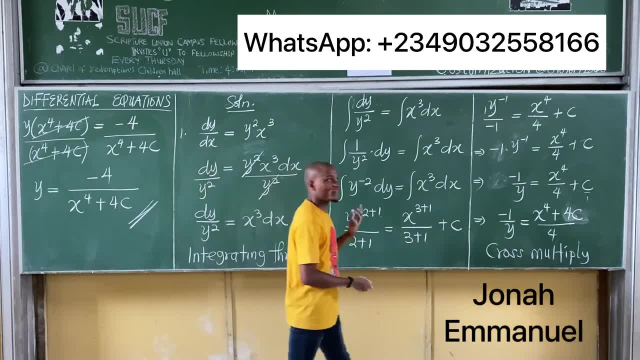 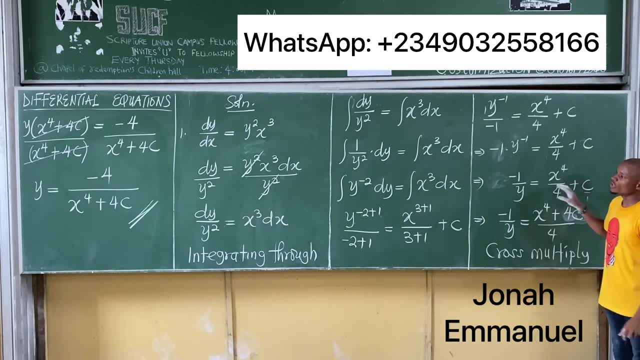 That becomes your answer. So here's the idea For the pressure equation. I will have stopped here. This 4 all over is okay, But you don't stop here, You only look. you look for a way to make sure that Y is not included, as in this case. 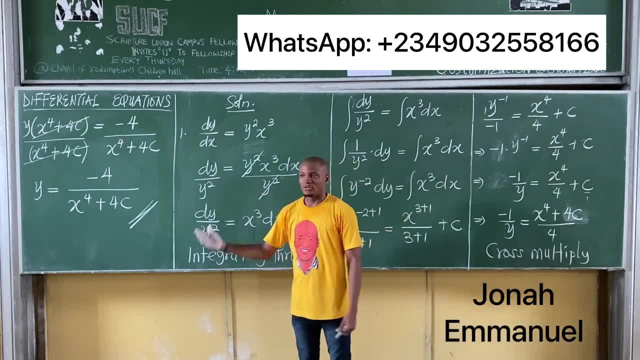 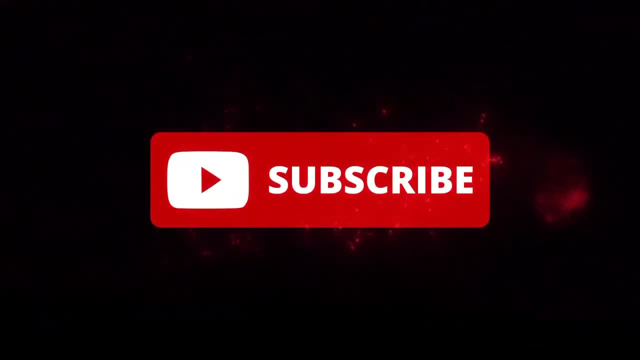 That's what you answer. This is how you answer this question.